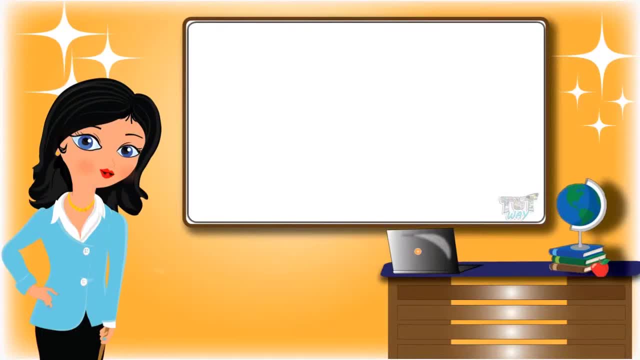 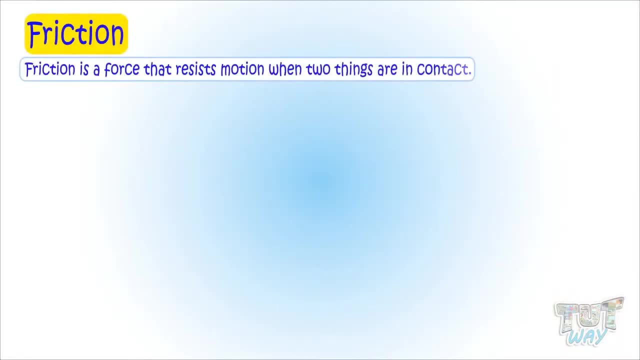 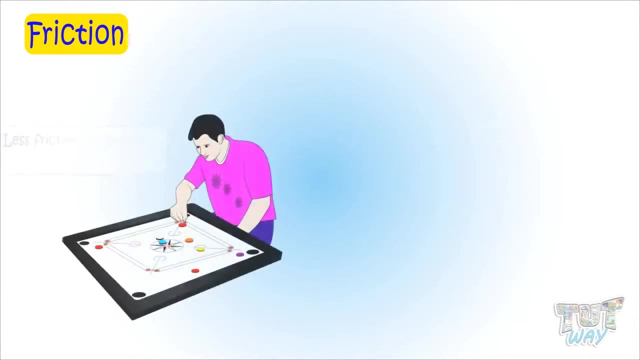 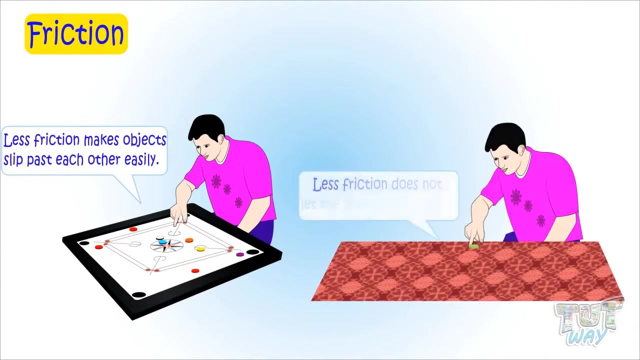 Hi kids, Today we will learn more about friction. So let's start. We learned that friction is a force that resists motion whenever two surfaces are in contact. When the friction is less, the objects slip past each other easily, and when the surfaces are rough, the objects does not move against each other easily. Example: 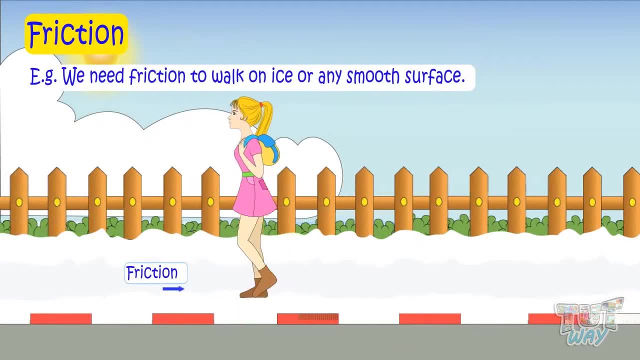 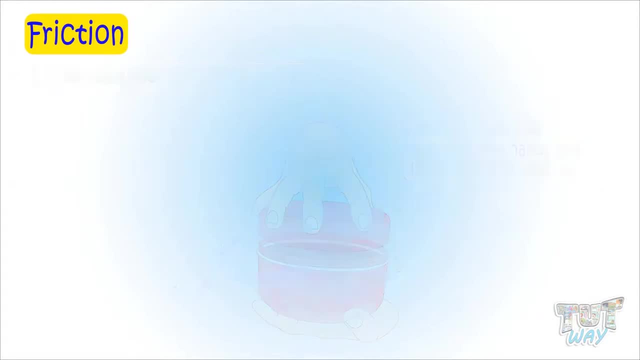 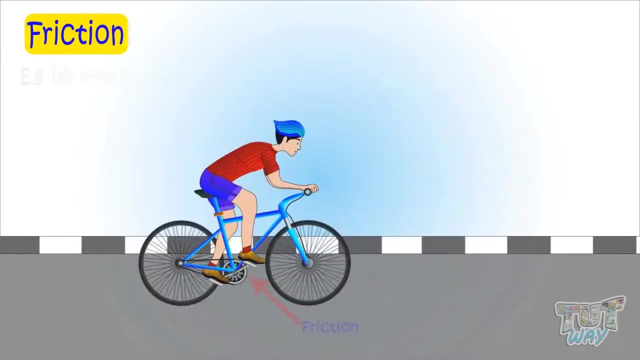 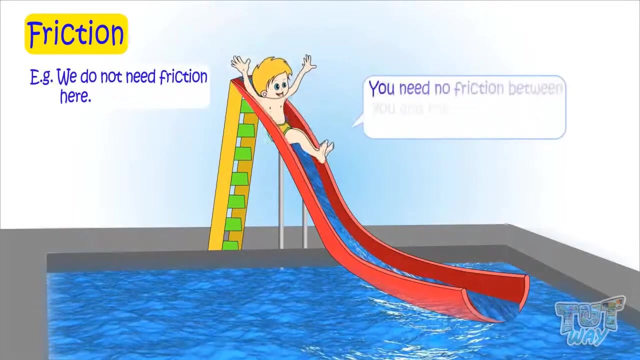 You need friction between your shoes and ice to walk on it. You need friction between your hands and lid of the jar to open it. You need grip between your hands and handle of the bicycle to hold it firmly. You need friction between your shoes and paddles of the bicycle to paddle it And you need no friction. 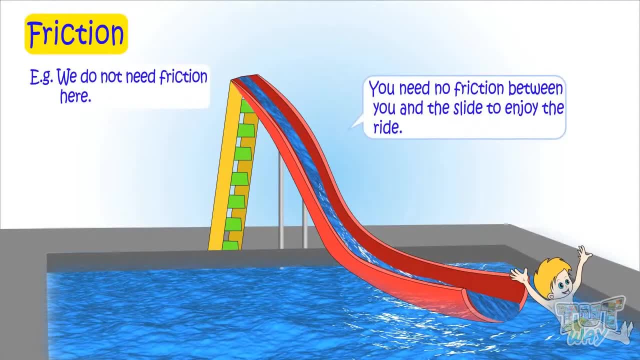 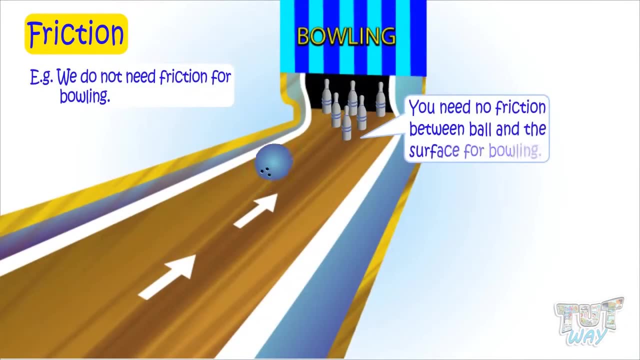 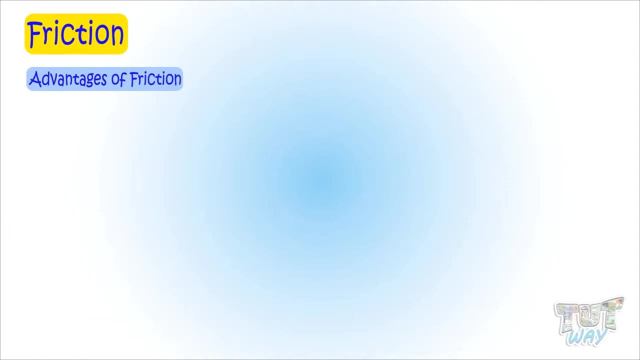 between you and the slide. to enjoy the ride, You need no friction between the striker and the board. to play, You need no friction between the ball and the surface for bowling. Now let's learn advantages of friction. Friction is very important while driving a car Without it. 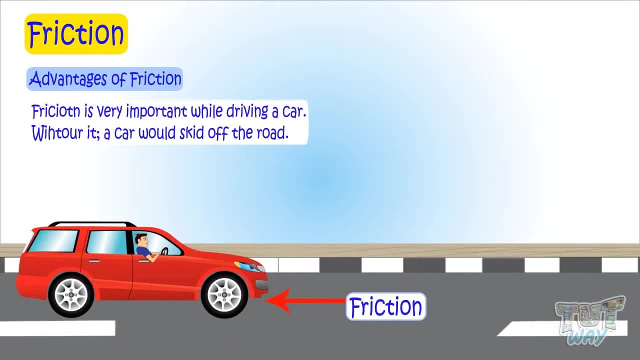 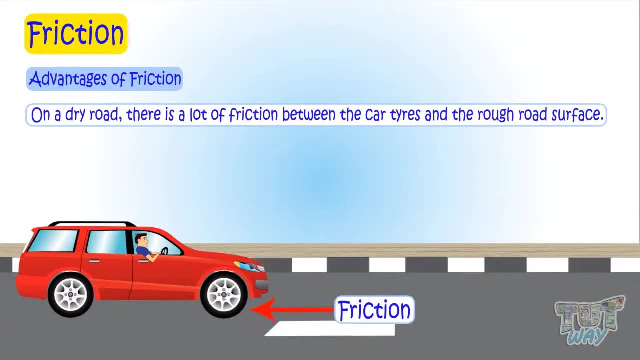 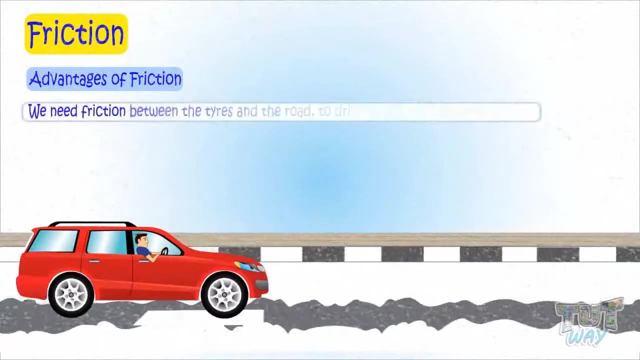 a car would slid off the road. On a dry road there is a lot of friction between the car tires and the rough road surface And in winters there is snow or ice on the road. That makes the surface of the road very smooth and there is little friction between the tires and the road. 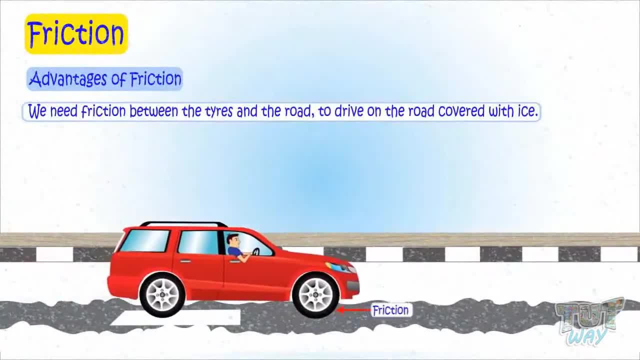 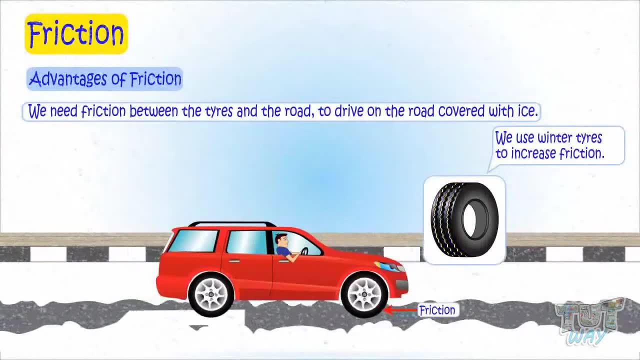 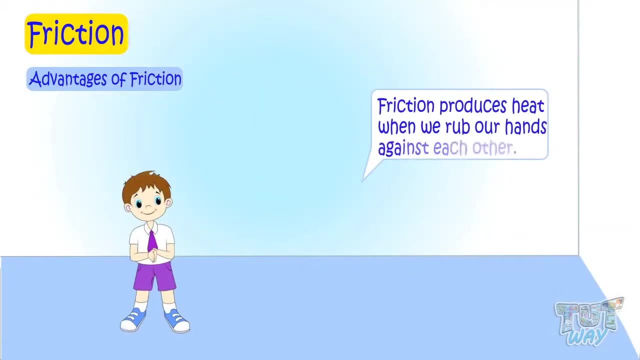 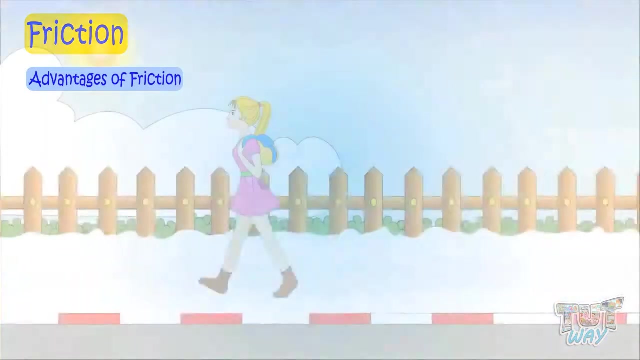 because of which the tires may slip off the road. This is why we need winter tires. Winter tires have special grooves to increase the friction in snowy and icy conditions. Friction also produces heat. When we rub our hands, it produces heat which warms our hands. Friction between 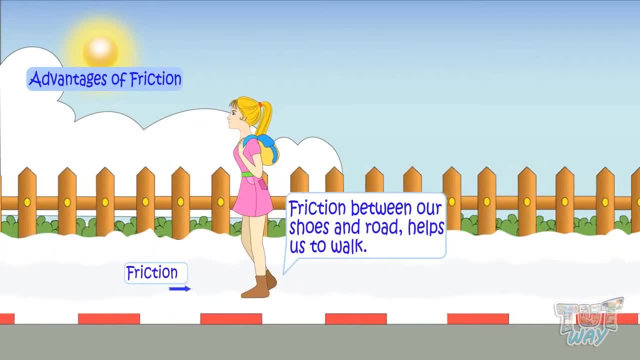 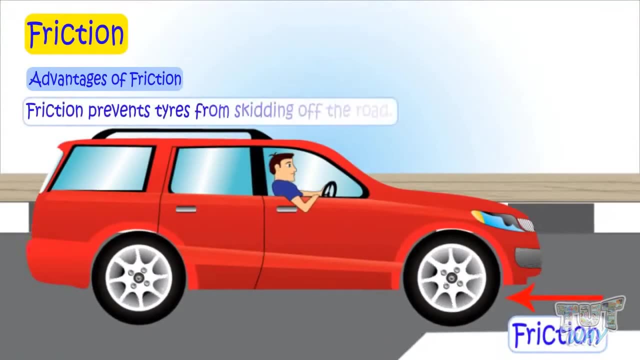 our shoes and road helps us to walk. Without friction, we will slip or fall. Friction helps to prevent the tires from slipping on the road, because wheels need friction to have grip on the road and move forward. This is the reason the tires have grooves: to produce sufficient friction.